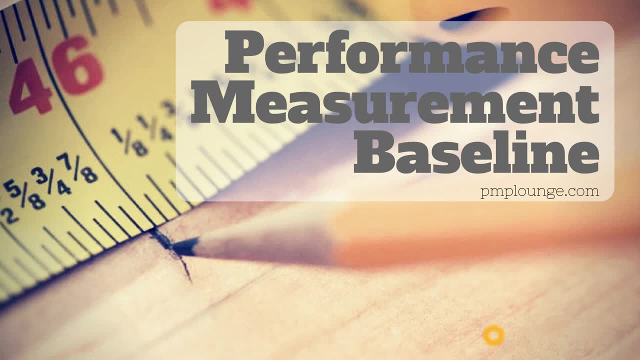 Hi and welcome to PMPLoungecom. Today we are going over a topic called Performance Measurement Baseline. Now, you are definitely going to come across this term in your PMP studies, So let's dive into it and try to understand. what exactly is PMB? 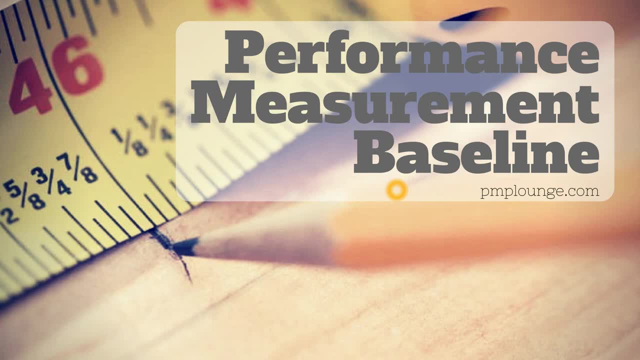 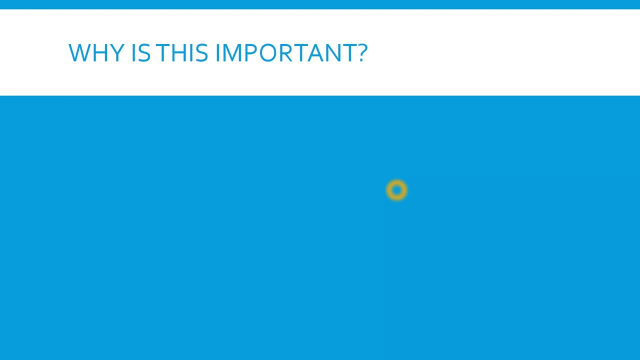 which is just the short form of the Performance Measurement Baseline. that is Alright. First up, why is this important? As always, this has been our favorite question before we discuss any of the PMB topics. Why exactly is this important? Why should you be studying and devoting some time for PMB? 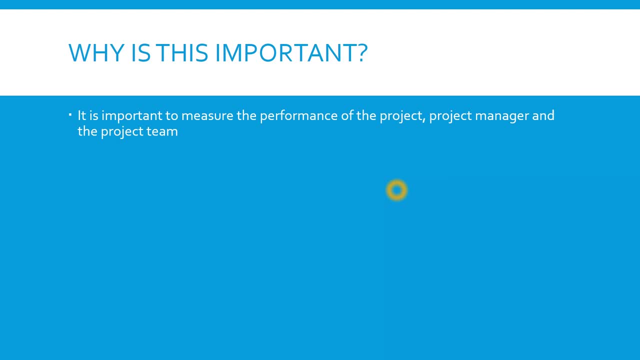 Well, first up in the real world, it is important to measure the performance of the project, the project manager and the project team. So you are doing a project, It's a six-month project. It's a six-month long project. 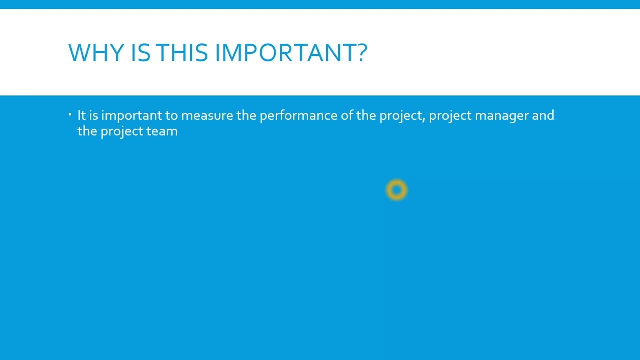 Two months later, if somebody comes up to you and asks you: Hey, how was the project going? What are you supposed to say? If you don't have any measuring stick, you will not be able to say how the project is going. 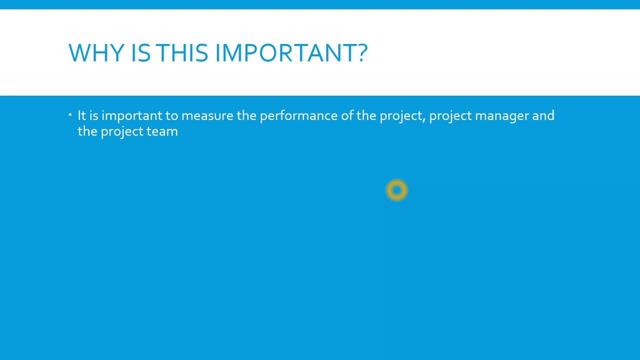 So, at each time, at each point of time, there is something that the project manager needs to do and needs to verify. There are certain benchmarks against which the project manager, the project manager, will verify where the project currently is. That my friend, is the PMB, by the way. 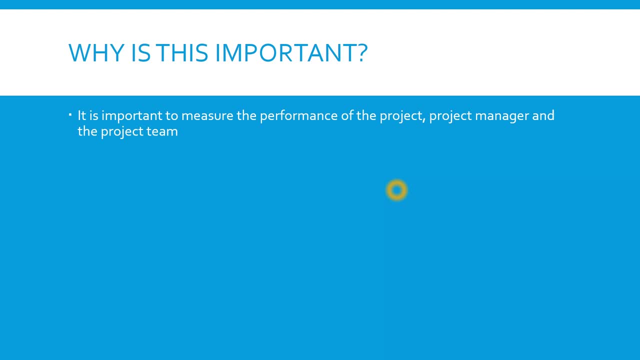 Okay, So project project manager, project team- everything needs to be measured. The performance of all three is important and needs to be measured, And the most prominent baseline which is used for measuring the project is the performance measurement baseline. So we said that it is important to measure the performance of the project. 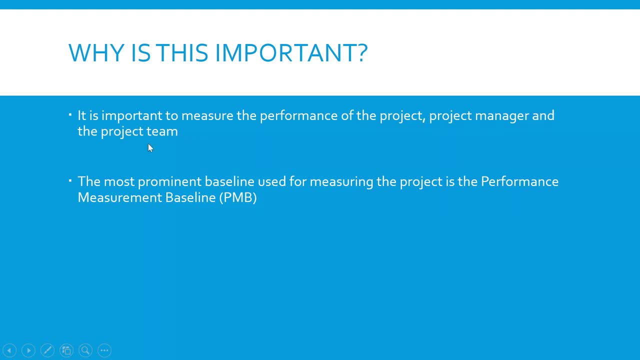 The project, the project manager, the project team- Not that project manager is different from the project team, by the way, But performance measurement baseline is basically something which you use to measure the performance of the project And, like I mentioned earlier, at any given point of time. 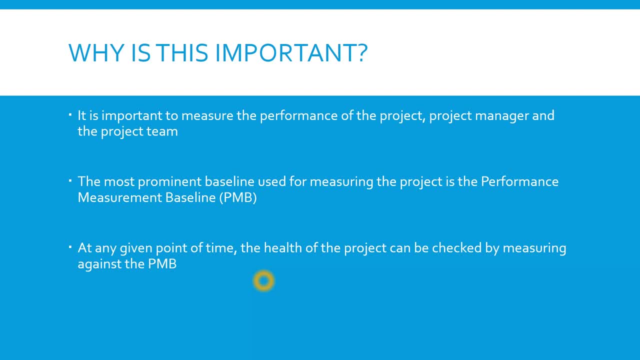 the health of the project can be checked by measuring against the PMB. So, like I said, a six-month-long project. two months later, if a stakeholder comes up and asks you how the project is going, you will pull out your PMB and measure your existing status of the project. 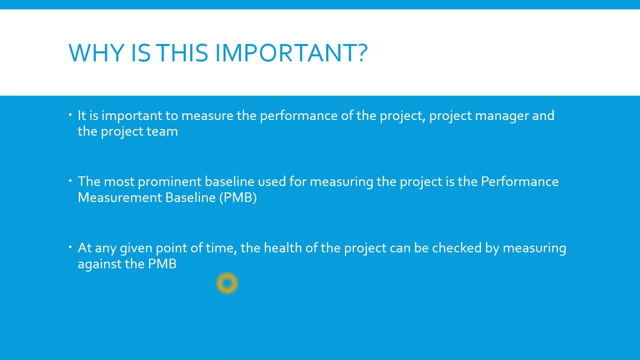 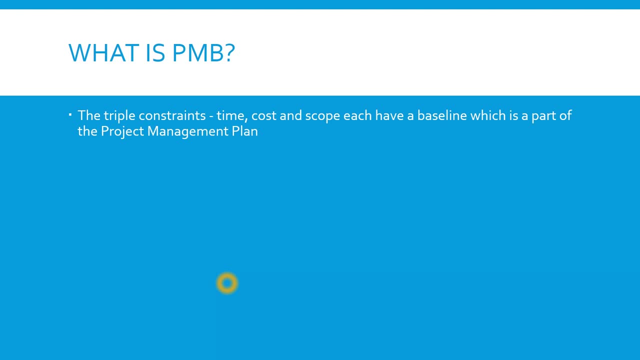 your current status of the project against the PMB. All right, Moving on Now, what the hell is PMB right? So the triple constraints, which are, of course, the time, cost and scope, which you already know by now. 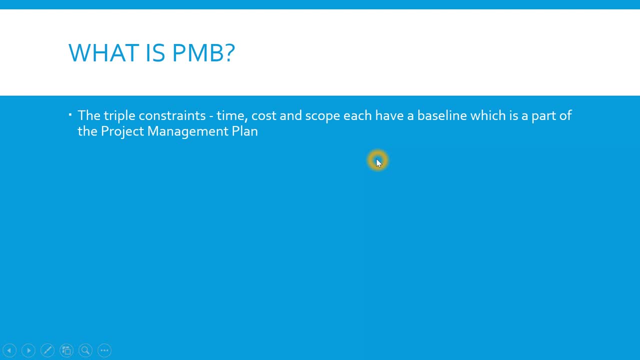 All have a baseline, which is a part of the project management plan. So there is a time, When it comes to time, we call it the schedule baseline. So, basically, there's a schedule baseline, there is a cost baseline and there is a scope baseline. 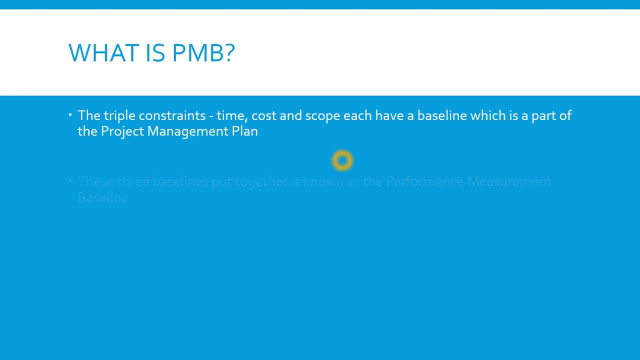 All of these are part of the entire project management plan. Now, these three baselines, the baselines of the triple constraints, which is the time, cost and scope put together, is known as the performance measurement baseline. So let's give it a. 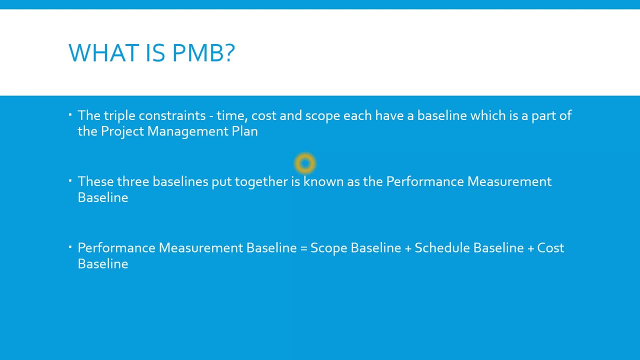 A mathematical tinge. Performance measurement baseline is equals to scope baseline plus schedule baseline plus cost baseline. Like I mentioned earlier, the baseline for time is known as schedule baseline. All right, So all three put together is what makes up the performance measurement baseline. 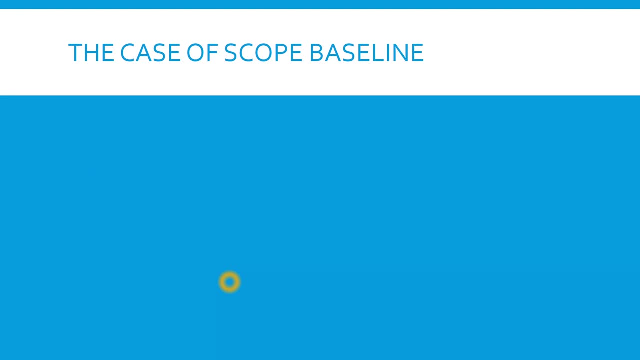 Now, something is different about scope baseline. What is that? So while schedule? So, while schedule, Schedule and cost baselines are just the final versions of the agreed upon schedule and cost, scope baseline is different. So scope is a bit different from schedule and cost. 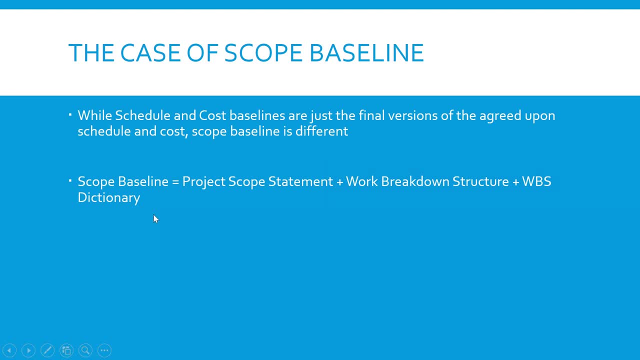 What is different in scope? This is what is different. So scope baseline is basically project scope statement. So there is a project scope statement, There is a work breakdown structure And then, to understand that work breakdown structure, there is a work breakdown structure. 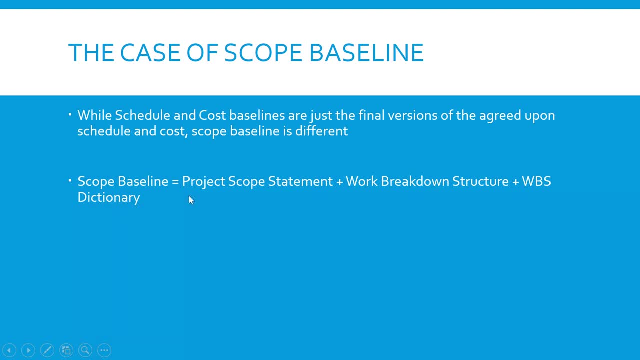 Dictionary, also known as WBS dictionary. So these three items together form the scope baseline. So, while schedule and cost baseline will be a single document, let's say, but scope baseline will comprise of three different documents: Project scope statement, work breakdown structure and WBS dictionary.